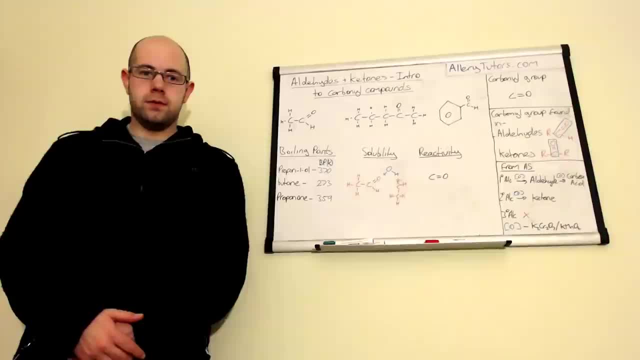 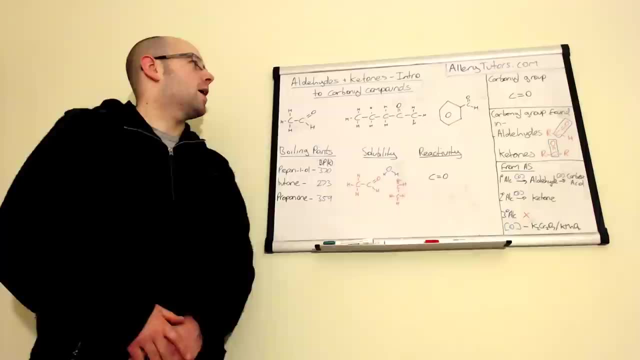 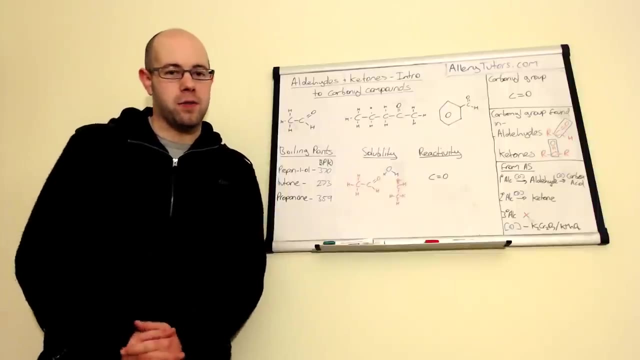 Hi everybody. my name is Chris Harris and I'm from Polymeretutorscom, and in this video we're going to look at aldehydes and ketones- and this is actually an introduction to the carbonyl group as well, or compounds containing the carbonyl group. So in this video we're 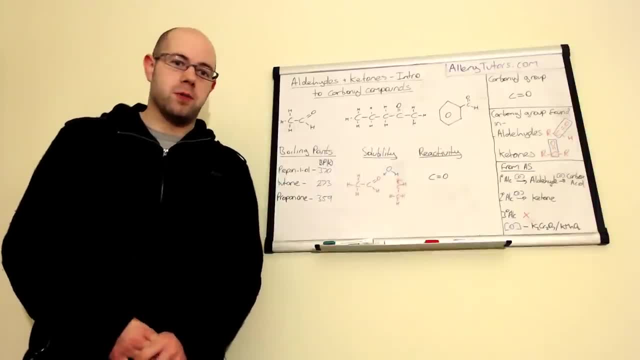 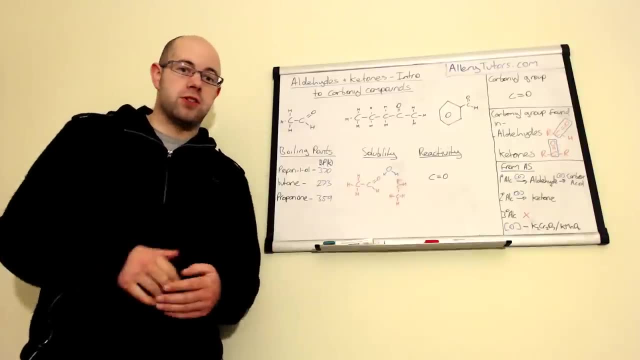 just going to do an introduction to some compounds that will have a carbonyl group fit in the molecule, and we're going to look at some of the key features of the carbonyl group in terms of solubility, reactivity and their boiling points as well. So we're going to 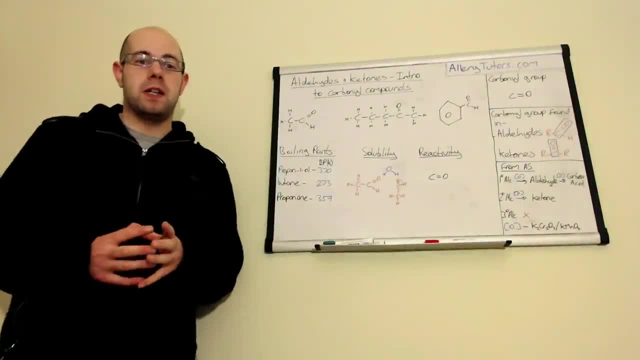 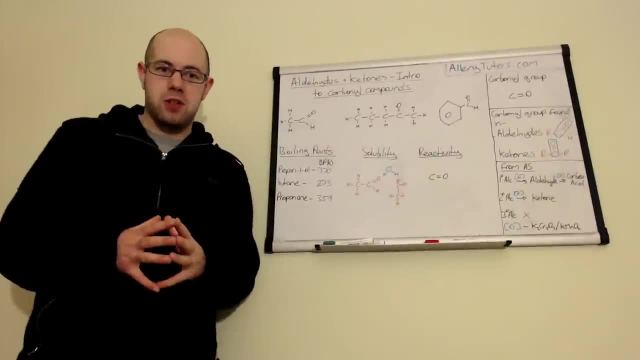 start with what the carbonyl group is. The carbonyl group is basically carbon with a double bond oxygen onto it, So it looks something like this, and there's a lot of molecules in organic chemistry that actually have the carbonyl group, and this could be, for example, aldehydes. 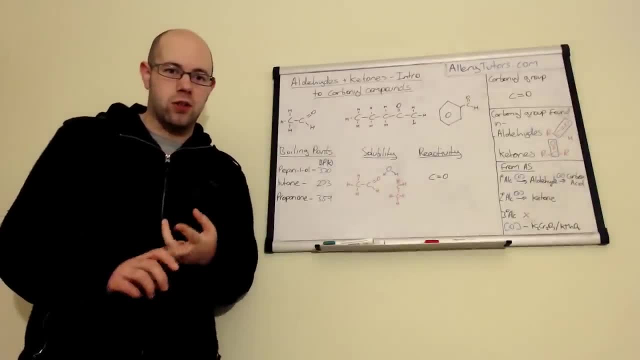 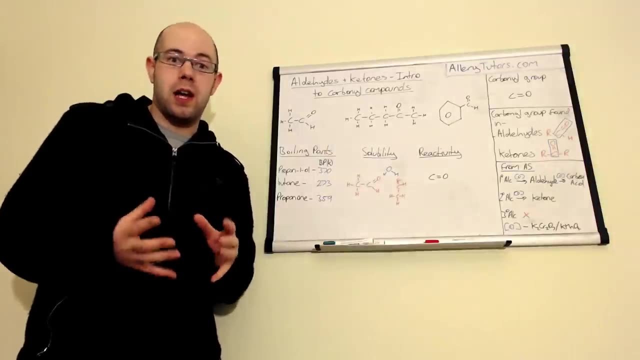 and ketones. You can also have esters, acid chloride, acetylcholine, So these are the acids that are carbohydrates, carboxylic acids, So there's loads of molecules in this, and so it will play a large part in organic chemistry. 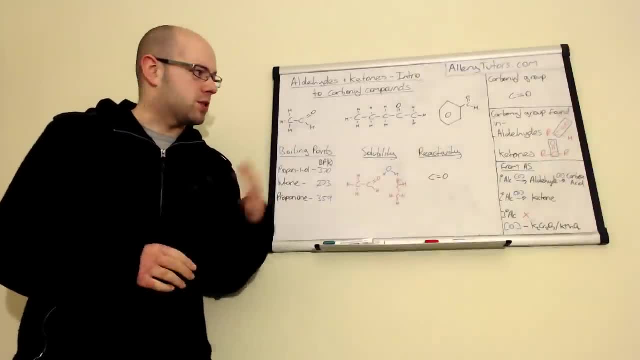 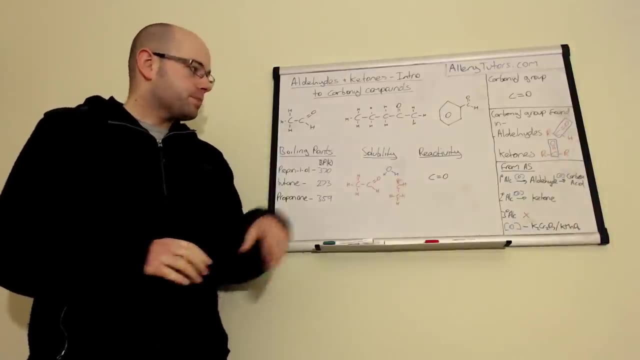 So we're just going to look at the first two for A2 chemistry, which is aldehydes and ketones, and we're going to look at what we can do with them and their reactions as well. So we're going to start with just looking at a bit of information from AS chemistry, where 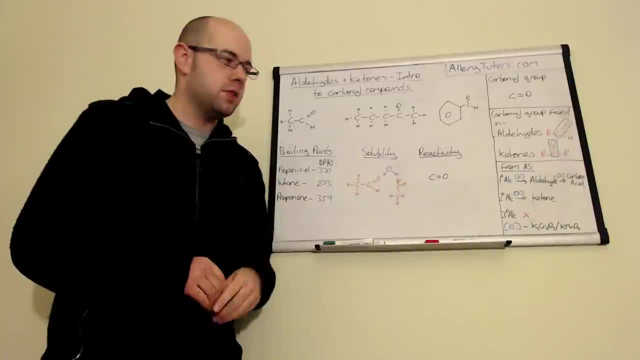 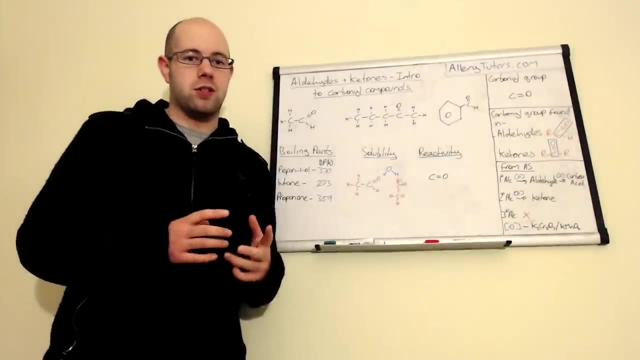 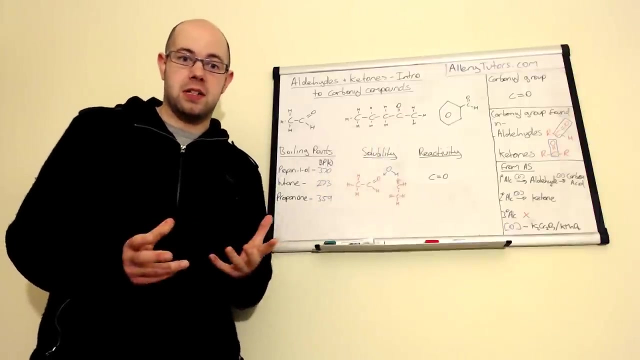 actually you would have looked at how you made aldehydes and ketones, and they're made from made from a primary alcohol and if you use an oxidizing agent such as potassium dichromate or potassium permanganate, then actually you can oxidize it to an aldehyde under distillation. 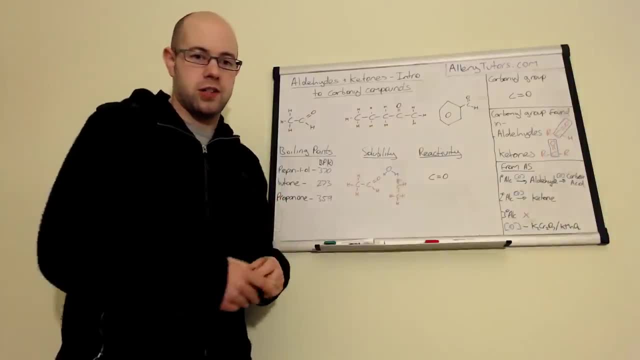 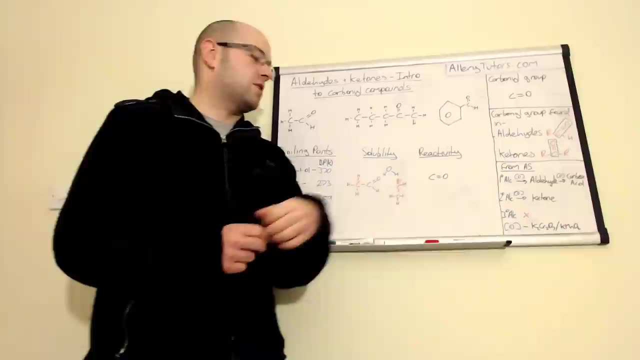 and if you were to oxidize it further under reflux conditions, then you can produce a carboxylic acid as well as the sage on the side there. And if you take a secondary alcohol and you oxidize that, you can make a keto. Tertiary alcohols don't oxidize at all, So it's just 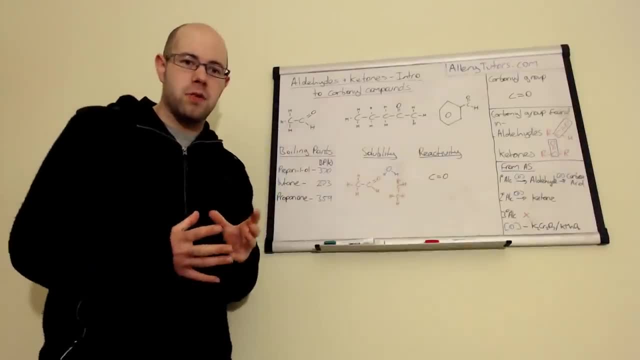 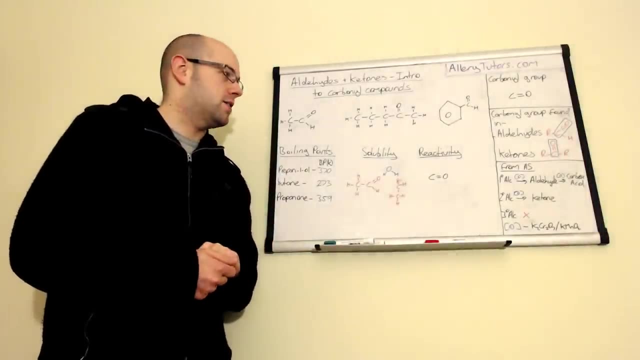 to show you where these aldehydes and ketones come from, and you do need to know the actual reactions regarding these as well, in terms of the reagents that you use and the conditions that you have to put them under. But we're going to start with here. So this is an aldehyde. 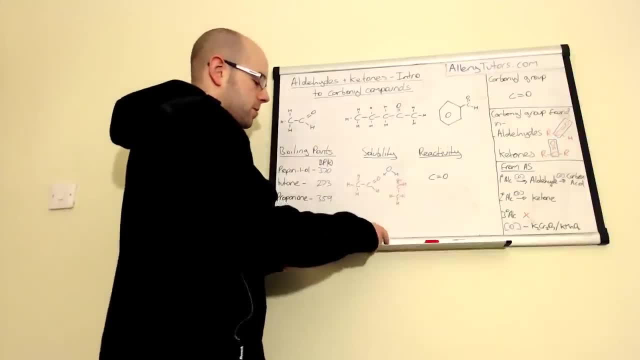 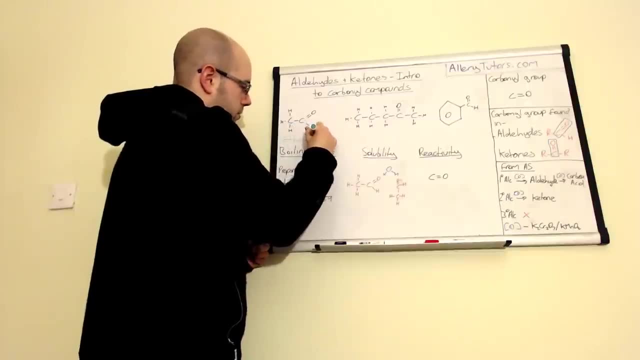 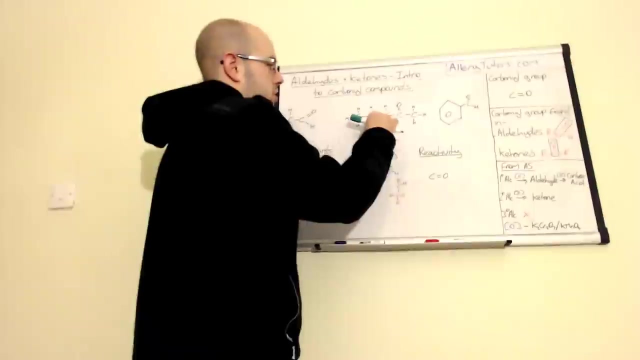 You are expected, obviously, to name these compounds as well. So this one is called because it's got two, so it's going to be ethanol, So let's put that one there. So that ends in L, because it's an L And we have a ketone over here. Now this one has got one, two, three, four, five carbons. 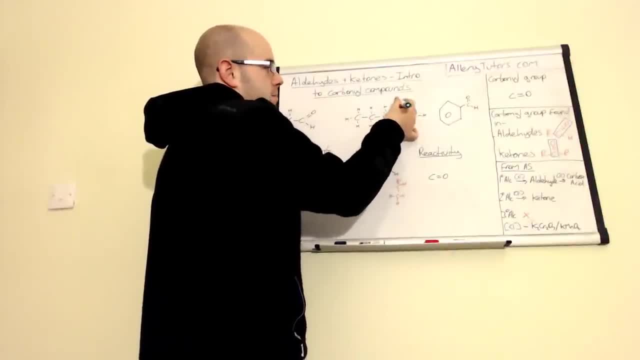 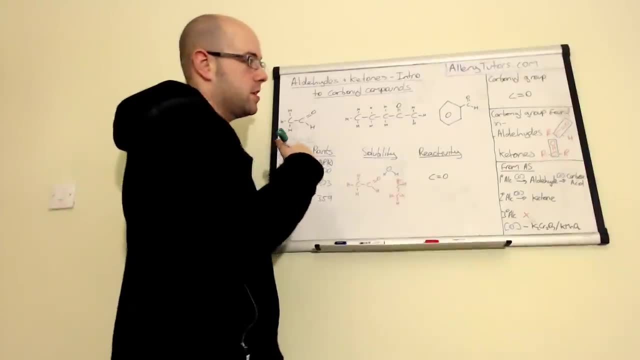 in there. So this one is going to be pent, But this has got a ketone in there, So it's still got your carbonyl group in there, except this one. the ketone is actually in the middle And we have to name where that ketone goes as well. So you can see that this is on the 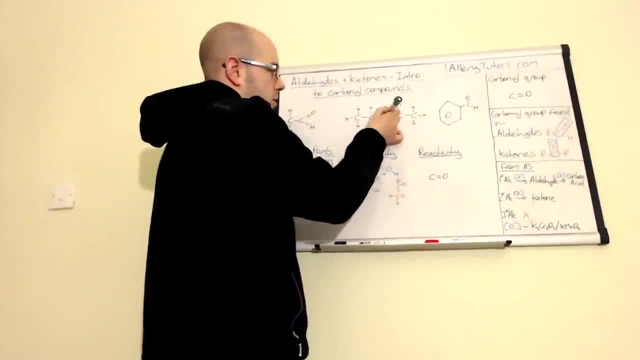 second carbon. If we number from this side one, two, three, four, five- then that's the lowest numbering combination that we can have. So if we start from here, that'll be one, two, three, four And obviously four is higher. 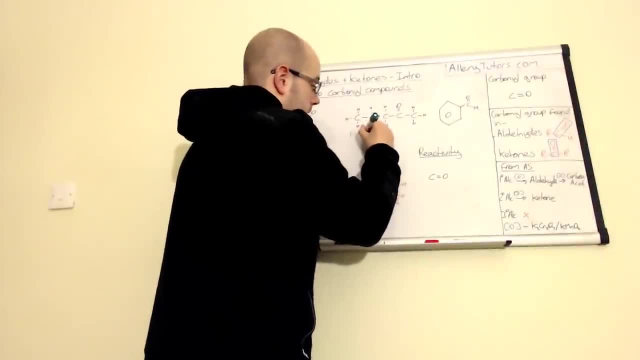 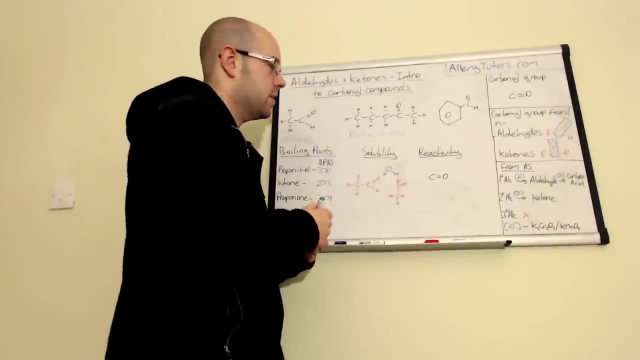 than two. So this is actually called pent, This is pentane And then two ole, And that shows that actually that group is in the second carbon. But you can, obviously you can have a different combination, where sometimes our carbonyl group might actually be in the middle. 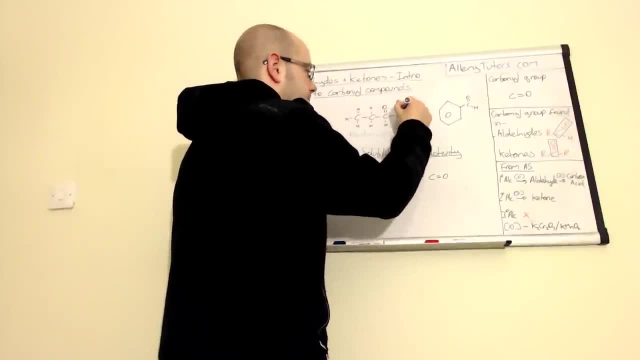 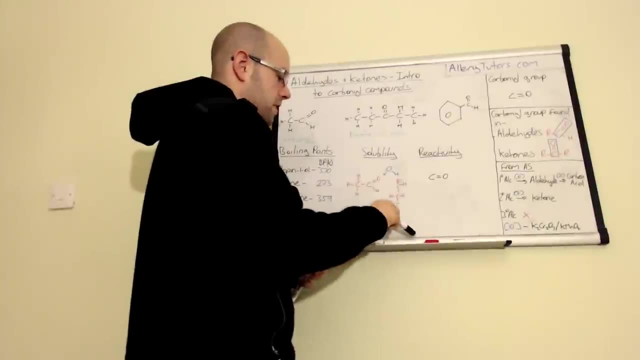 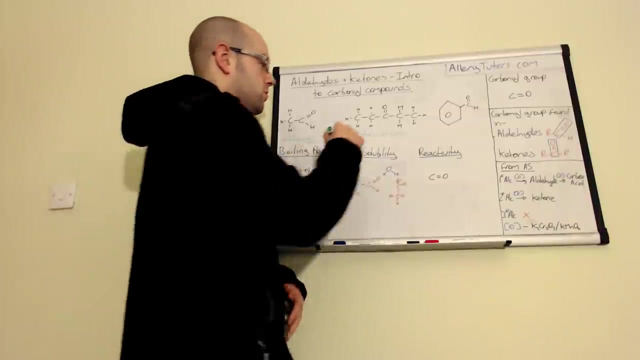 carbon, So we'll put that in there. instead, We'll put our hydrogen there And the hydrogen there, And this actually changes the name of it. So this is an isomer, what we call a positional isomer. A positional isomer because we're changing the position of the functional. 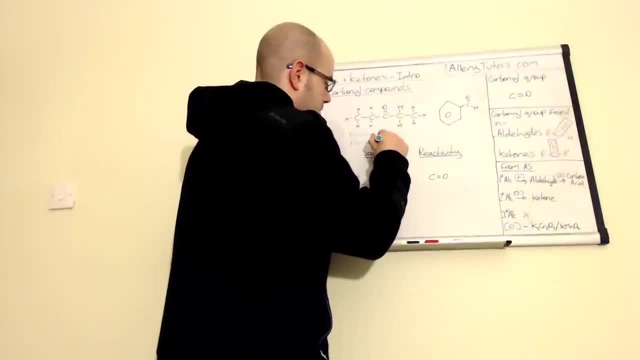 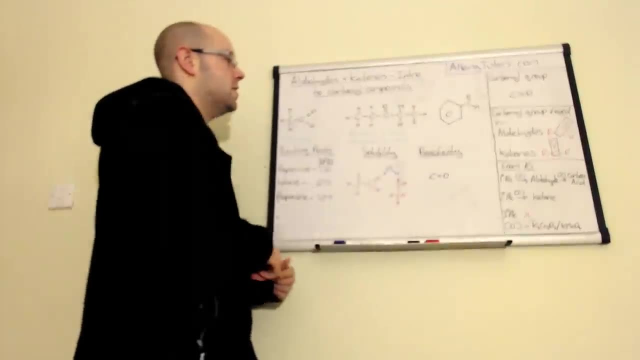 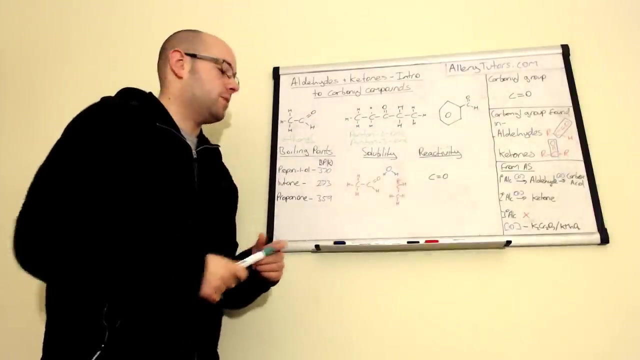 group. So this one is still pentane because it's still got five carbons, But this time this one's three ole. If it was on the end, obviously that won't be a ketone, That would be an aldehyde, because aldehydes are always having a carbonyl group on a terminal carbon. 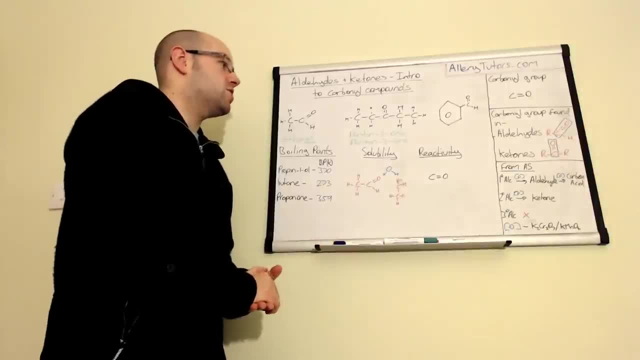 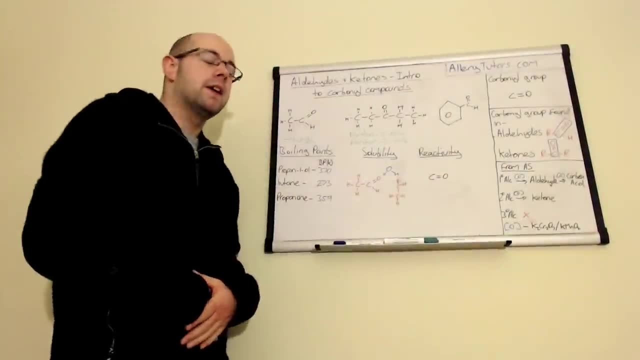 on either side of the molecule, Because it's A2,. there are topics that look into aromatics as well as arenes, And this is an example, which is benzene. Now there is a new way of naming this: This, if we have. 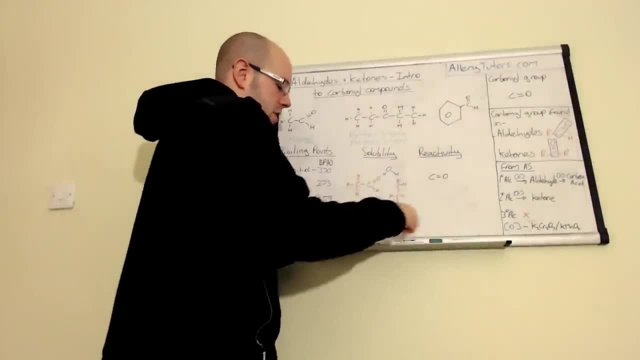 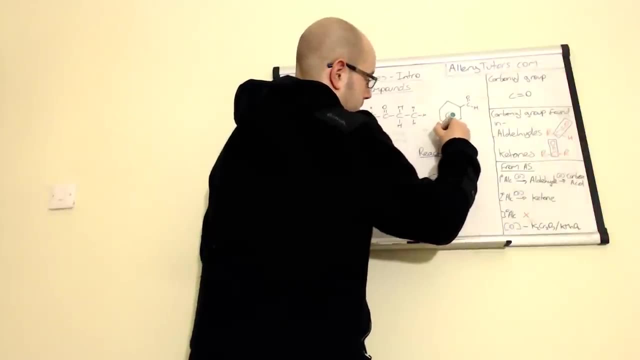 an aldehyde on the end of our benzene molecule. we actually give it a new name, And I'll write this one in green as well. So we start with benzene. So I'll put that there, And actually we have a new substance. 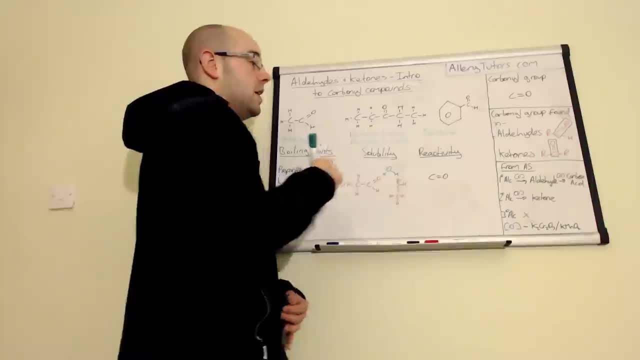 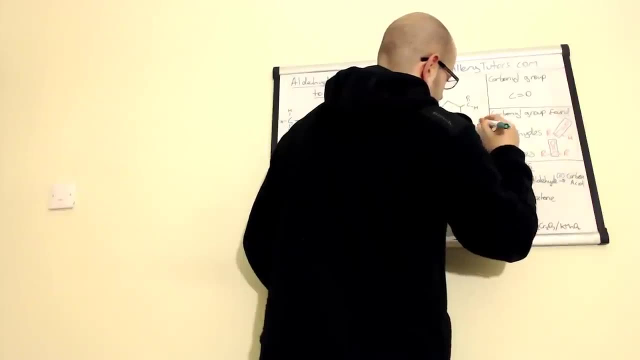 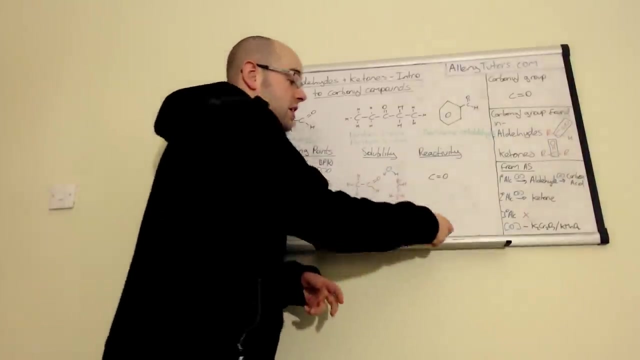 We have a new substance to add onto it. So when we have an aldehyde connected on the end, we call it a carbaldehyde. So benzene we call it carbaldehyde, And this is actually the new way of actually naming it, which you might not have seen before, But just be aware. 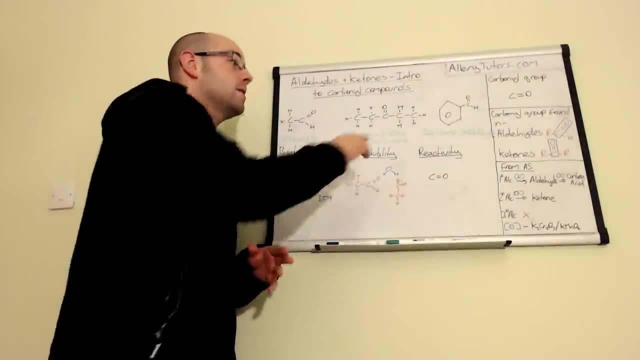 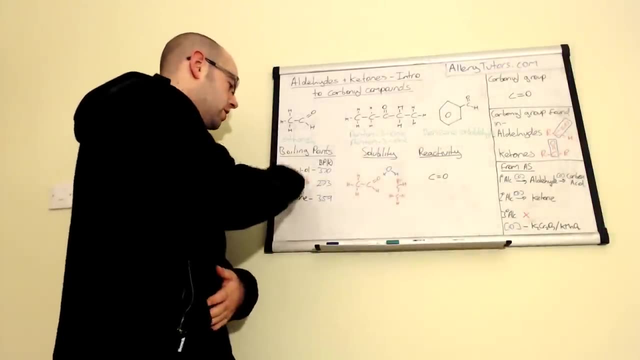 that if you have an aldehyde attached to a benzene ring like that, then that's what you should end it as- as benzene carbaldehyde instead. Right? So if we look at our next one here we're just looking at again, comparing aldehydes- 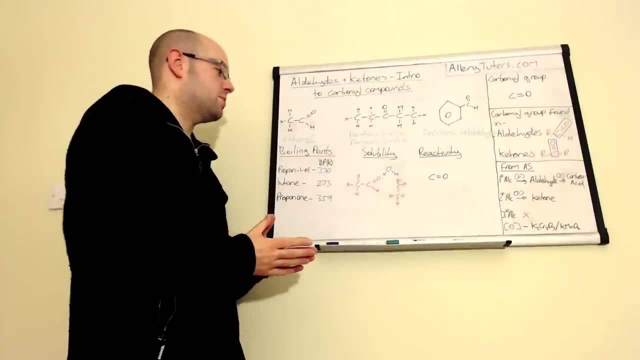 and ketones with other molecules and looking at the forces that's actually between them. So we've got three different molecules here. All have very similar MRs And so hence their van der Waals forces between the molecules of each of these are roughly the same. pretty, 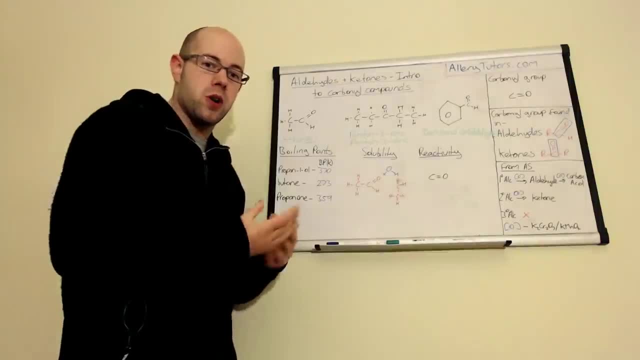 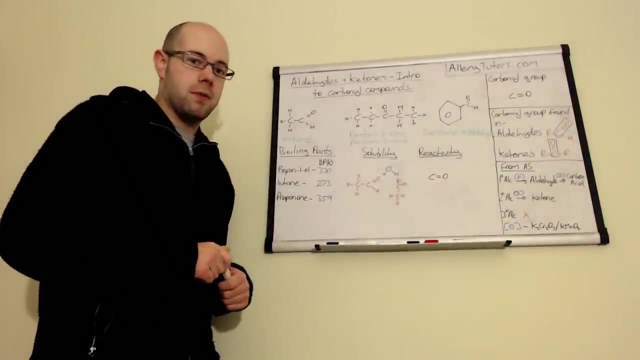 much. So any difference in boiling point has got to be because of other intermolecular forces. Now we're just going to write next to them what type of intermolecular forces are in these. So we've got propan-1-L, which is the strongest type of intermolecular force. So they all. 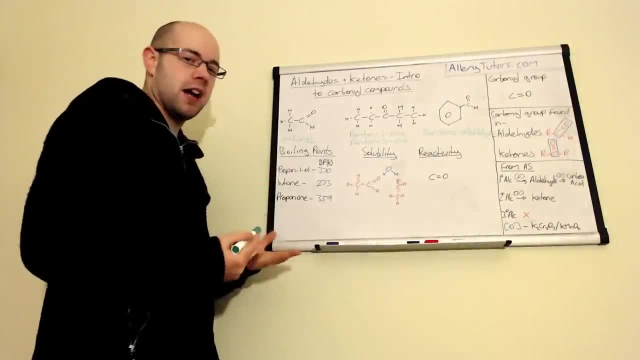 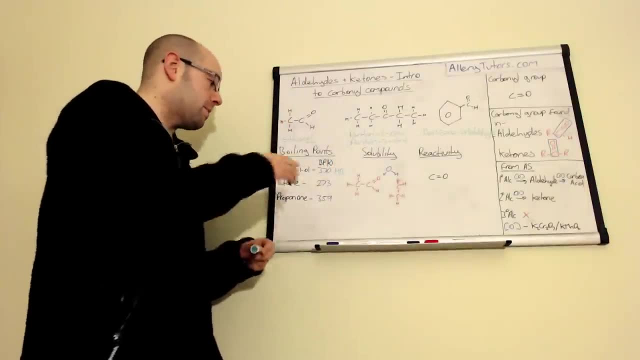 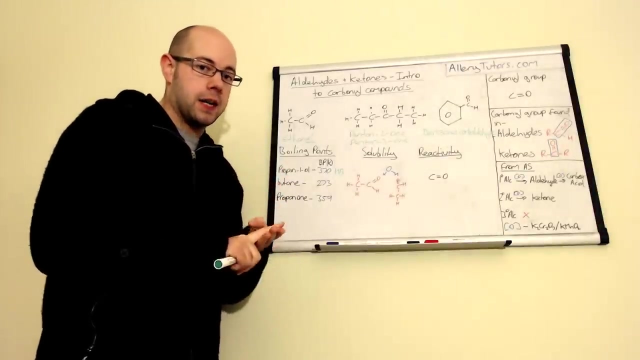 have van der Waals And propan-1-L is an alcohol. So alcohols actually have hydrogen bonding as their strongest intermolecular force. And remember, propan-1-L will actually have. it will have all three intermolecular forces. It will have van der Waals, dipole-dipole. 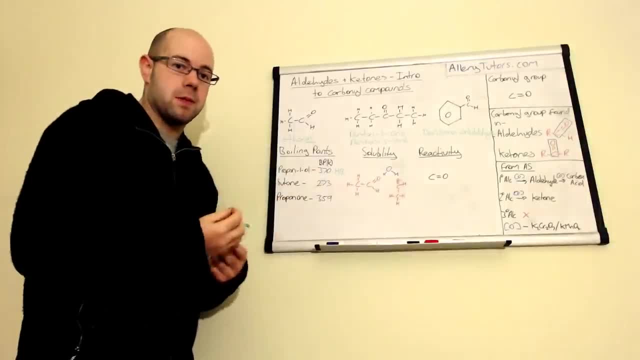 and hydrogen bonding, And so the hydrogen bond is the strongest intermolecular force that this has. Butane is just a bog standard hydrocarbon. So butane actually all that has is van der Waals Right. So it's a very strong intermolecular force. So it's a very strong intermolecular. 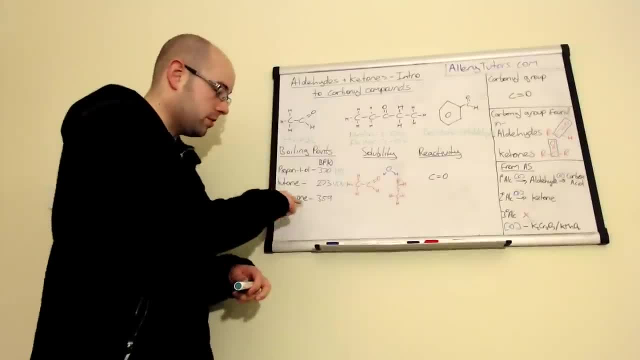 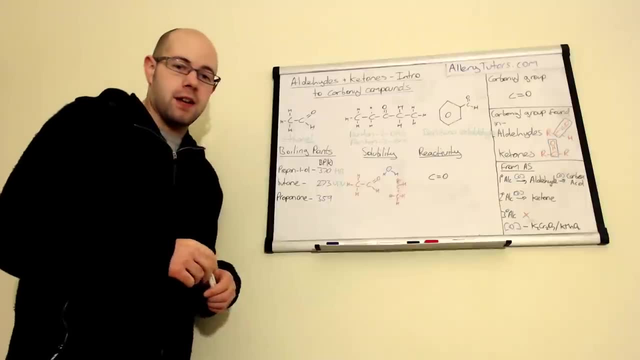 force, The van der Waals forces, so put VDW And propanone can't hydrogen bond with another propanone molecule. But what it can do is it can interact via a dipole-dipole. So I'm just going to put DD, which goes there, And that shows it's dipole-dipole interaction. 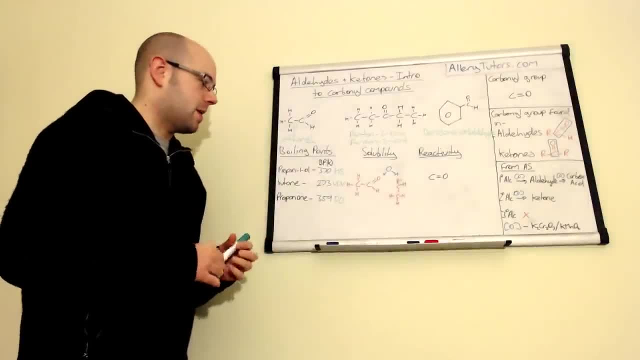 Now, in terms of strength, you may remember from AS chemistry that actually the van der Waals force is the weakest force And the dipole-dipole is the one that's in the middle And your hydrogen bond is actually the strongest intermolecular force. 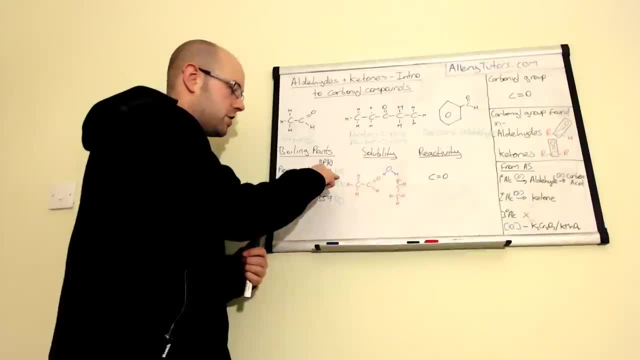 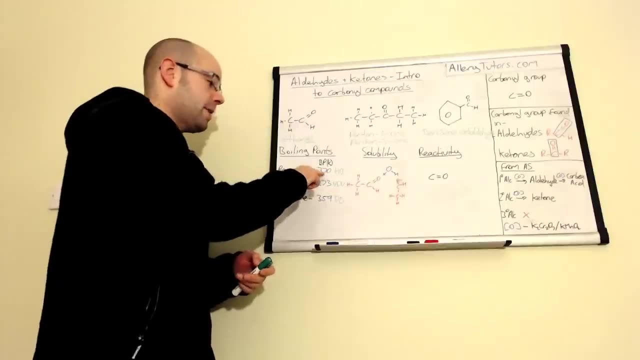 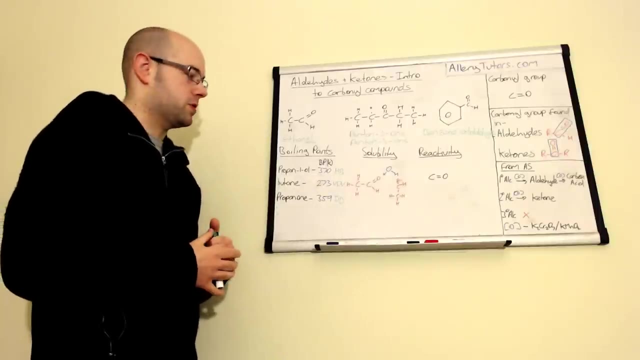 So molecules with hydrogen bonding and the same level of van der Waals will actually have the highest boiling point, And that's what we can see there. So propanone monol is 370.. Our propanone is 359, slightly lower because its strongest intermolecular force is a dipole-dipole. 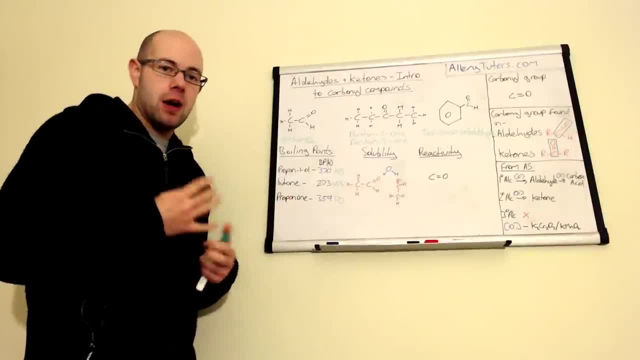 And you can see that butane is actually quite a way behind. All butane has is a van der Waals force. It doesn't have anything else, And that's the strongest intermolecular force. So it is important to be able to compare these And these interact. these molecules interact. 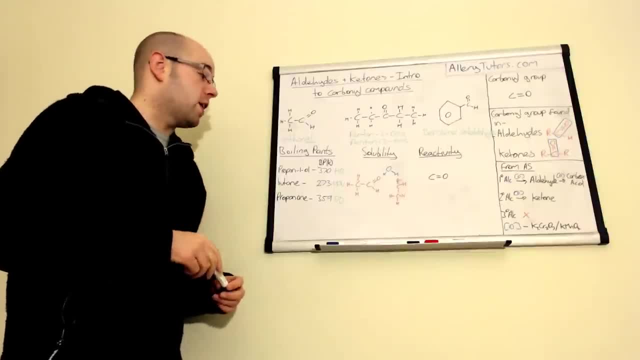 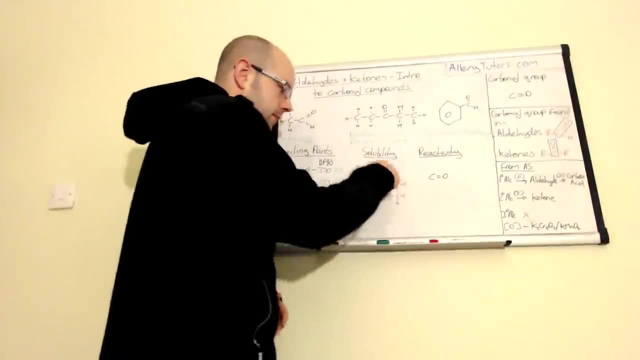 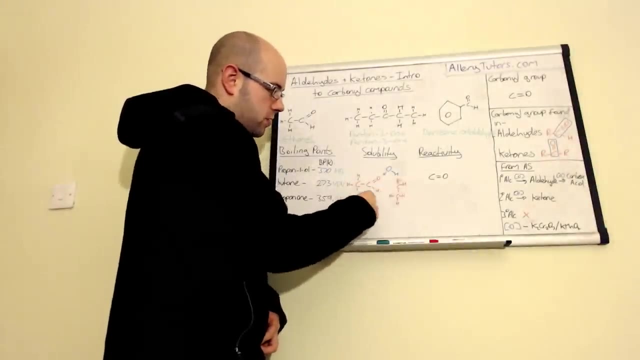 by a dipole-dipole, But when it comes to actually dissolving with water, they can actually bond with water in terms of a hydrogen bond. So I've got a water molecule here And this is going to look at the solubility. I've got two aldehydes here which are at the end. 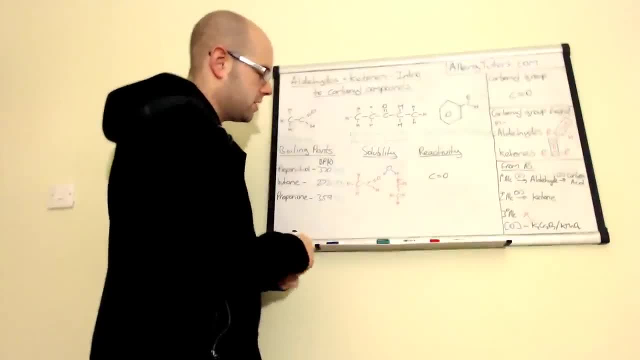 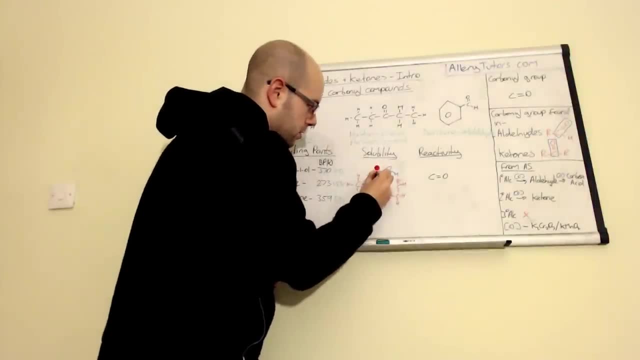 And I'm just going to show you how they interact So you can see. here's your solubility And oxygen. And the oxygen will have a lone pair of electrons. So it's got a lone pair of electrons on that oxygen. there It'll actually have two, but we're only going to draw one. 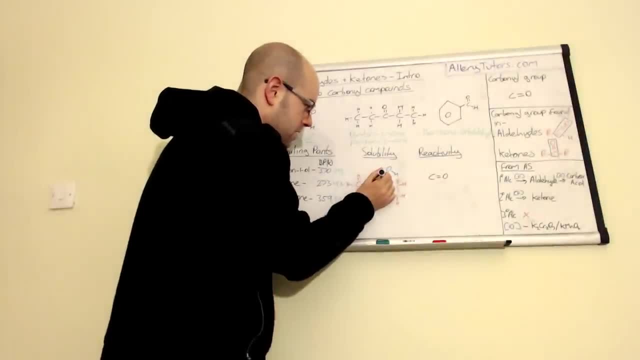 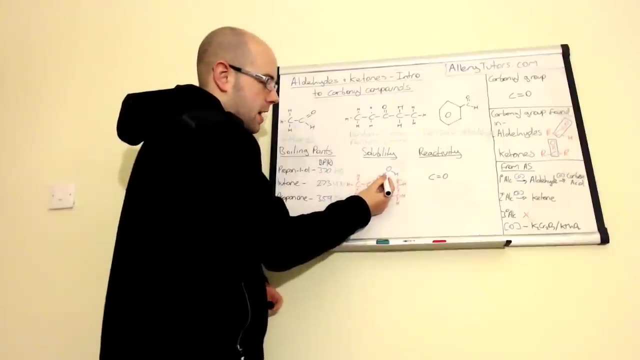 because that's how it's interacting, And you can see that actually what we have is a small hydrogen bond that occurs between the lone pair of electrons on the oxygen and the delta positive hydrogen. So I'm going to put a delta positive on there And so that little interaction. 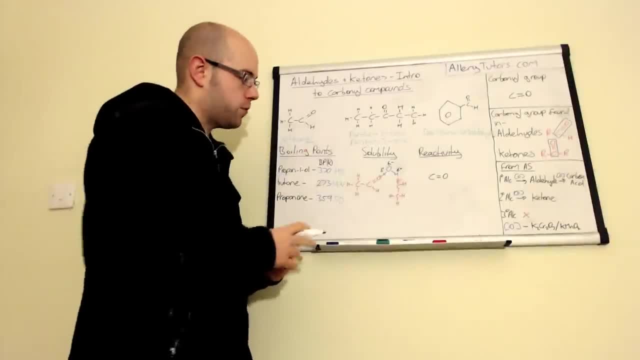 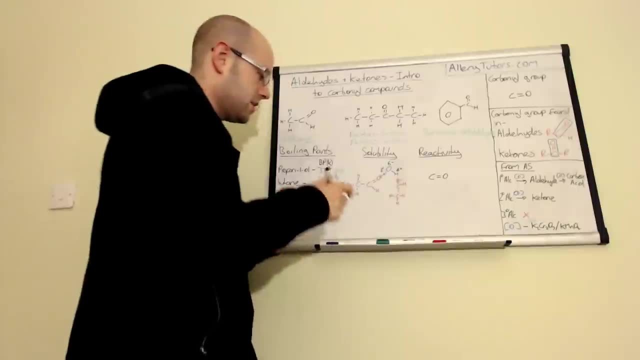 there is actually a hydrogen bond, And if it can form a hydrogen bond, it's going to form a hydrogen bond with water. We can effectively say that these are relatively soluble. They can dissolve quite easily, And it's likewise. it's the same on this oxygen here, on this. 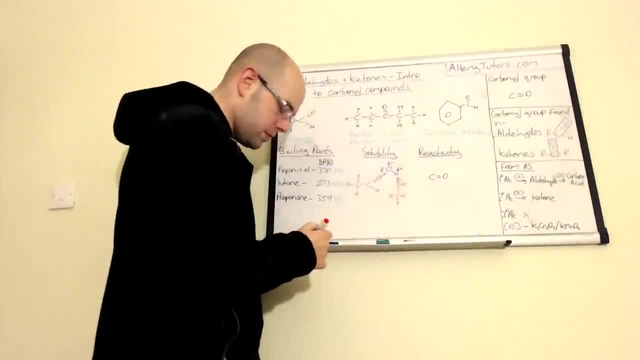 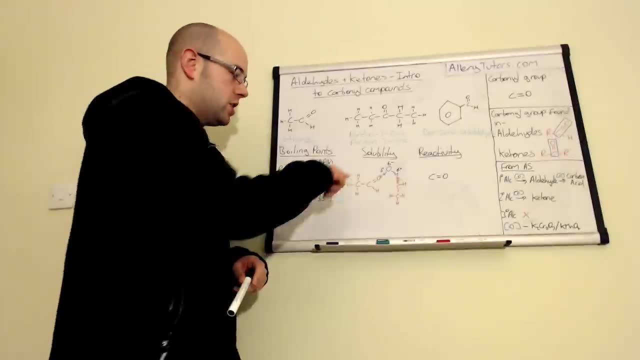 other aldehyde on this other aldehyde as well. Ketones behave in a similar way as well. They will dissolve. They're quite soluble as well, And it is important to know that actually the larger the aldehyde or the bigger the MR, the more insoluble it is. So mainly 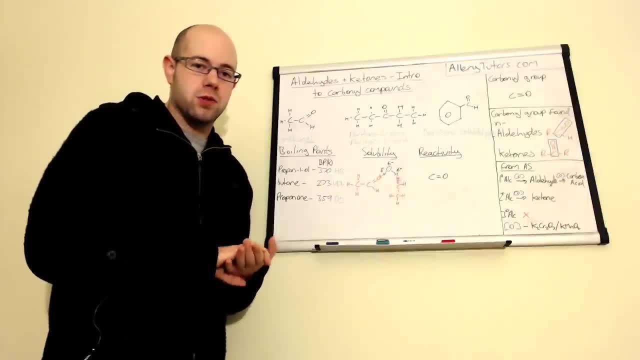 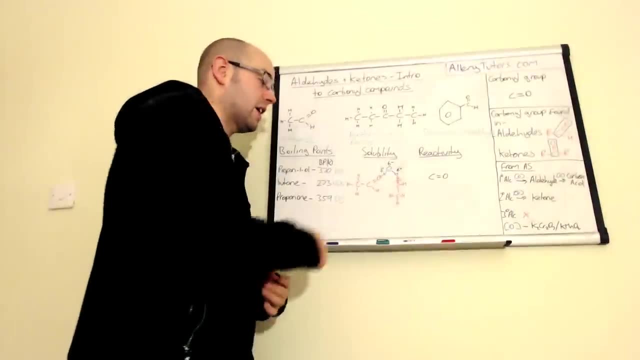 it's only your shorter chain, aldehydes and ketones, which will actually dissolve, And but the longer the chain, the less soluble they are, And mainly because it's only this bit that's actually soluble. If you have a big, long, insoluble hydrocarbon chain, it will struggle.